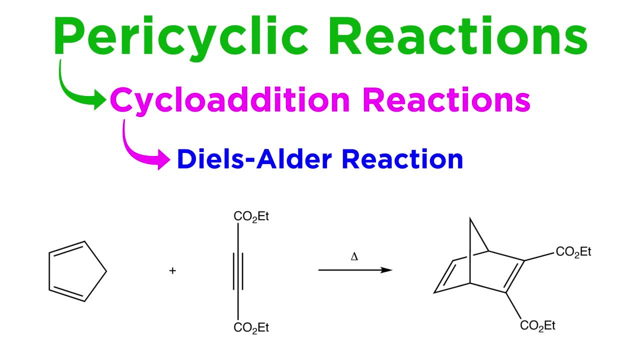 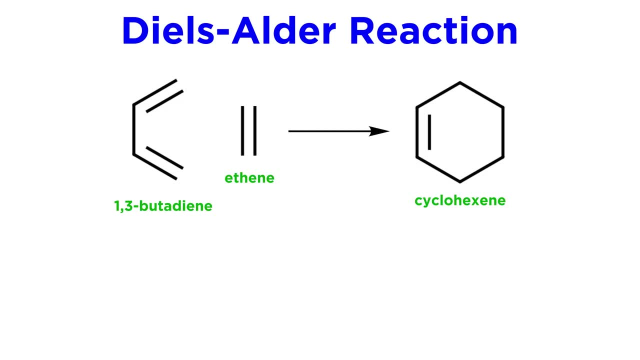 so, to start from a familiar place, let's revisit the Diels-Alder reaction and dig a little deeper. Looking at the simplest possible Diels-Alder reaction, we have 1,3-butadiene and ethene, which react to generate cyclohexene. As we recall, any Diels-Alder reaction will. 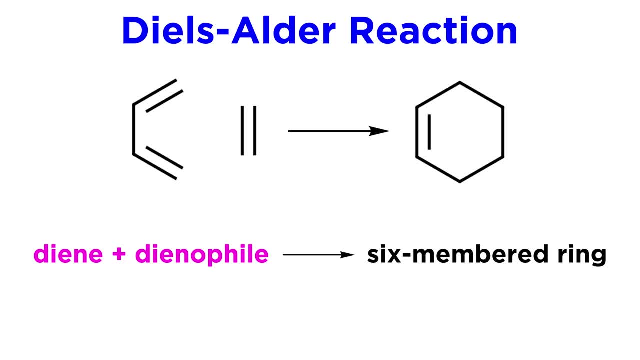 follow this basic setup, with a diene and dienophile going to generate a six-membered ring with a pi bond. The mechanism for this reaction is in stark contrast with just about any other reaction we have investigated. Typically, when a chemical reaction occurs, there is some electron-rich species that interacts with an electron-poor. 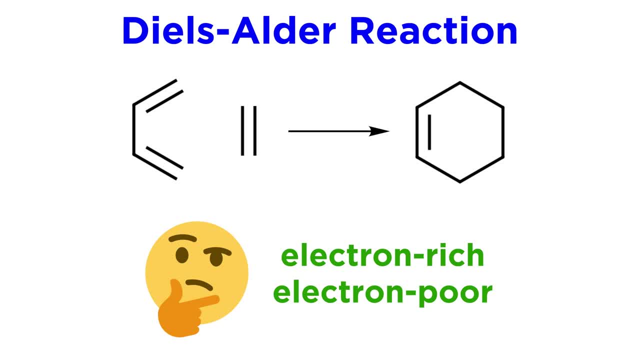 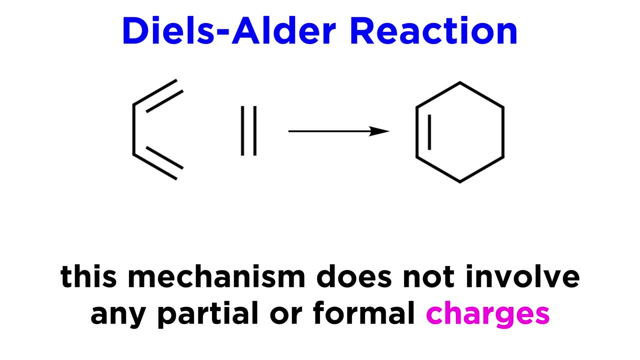 species, like when a nucleophile attacks an electrophile or an acid-base reaction. but here we see no such things. There are no polar bonds and there is no intermediate. The reactants combine through a simple transition state with no charges or dipoles. This is a 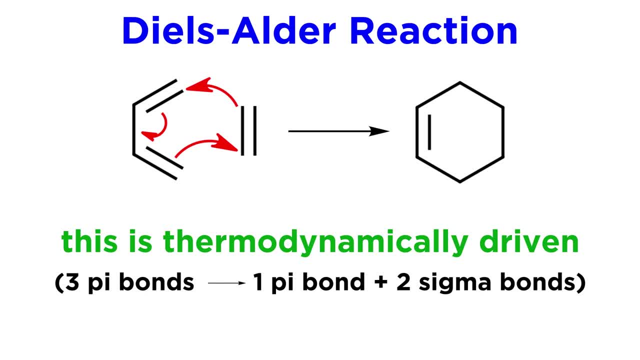 dynamically driven reaction based on the stability of sigma bonds over pi bonds, given that three pi bonds go to form one pi bond and two sigma bonds, which occurs under appropriate thermal activation, meaning above a certain temperature. In displaying this mechanism, we must understand that these arrows are not to be interpreted literally. the pi electron density. 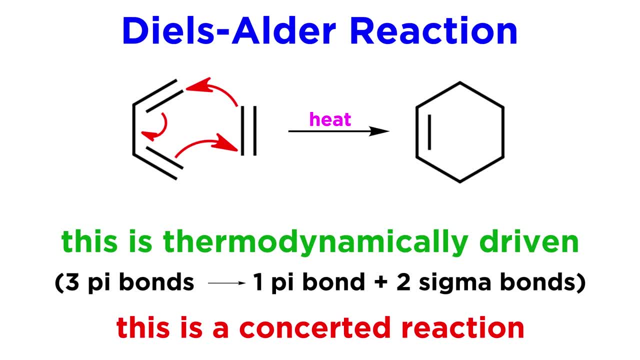 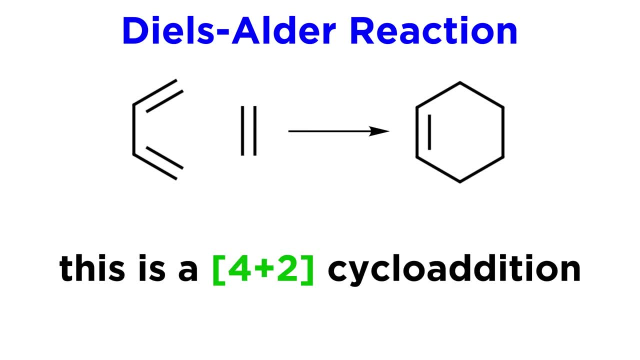 does not cyclize in a specific direction. The pi bonds dissipate as the new bonds materialize in concerted fashion. We should also understand that the Diels-Alder reaction is a 4 plus 2 cycloaddition. This means that the diene contributes four pi electrons and the dienophile 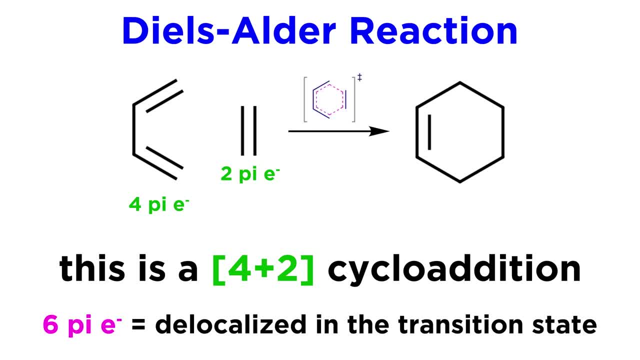 contributes two And these six pi electrons that are involved in the cyclization. these are the electrons that are delocalized in the transition state. We could then wonder what other types of cycloadditions are possible. Can we do 2 plus? 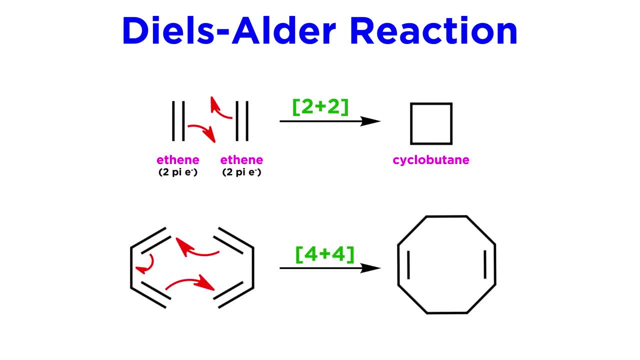 2? Or 4 plus 4, as well. We could imagine ethene reacting with itself to form cyclobutane, Or this diene reacting with itself to produce this cyclooctadiene. But in fact these reactions do not. 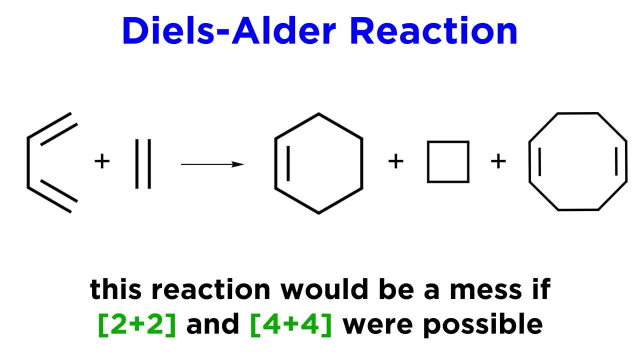 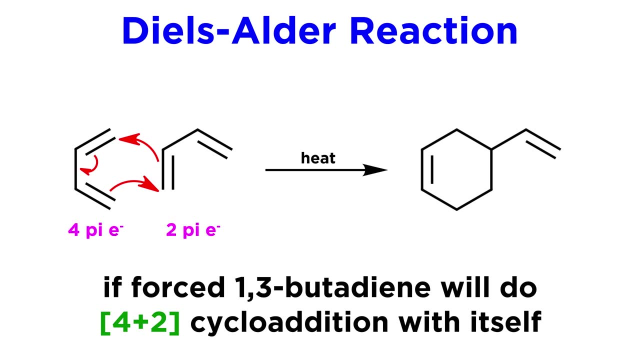 occur thermally. This is quite good, as otherwise the Diels-Alder reaction between these two compounds would yield a messy mixture of products. In fact, if 1,3-butadiene is forced to react with itself under extreme conditions, it will still perform a 4 plus 2 cycloaddition, to give. 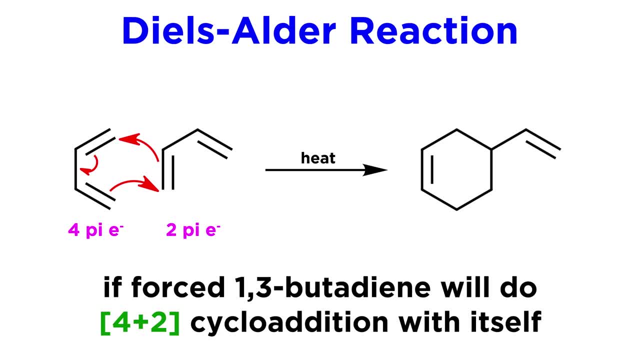 this Diels-Alder product, breaking the conjugation of the diene in the process, But never a 4 plus 4.. So what is it about the 4 plus 2 combination that works where the others don't Much like? 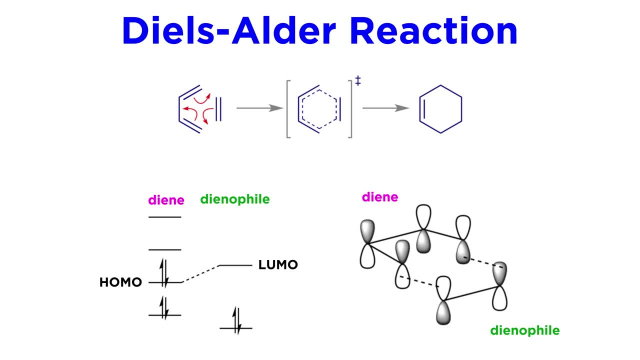 many other chemical phenomena, the explanation involves molecular orbitals. We did touch on this in the introductory tutorial regarding Diels-Alder reactions And we understood that in order for the highest occupied molecular orbital of the diene to put electron density into the lowest unoccupied molecular orbital of the dienophile, 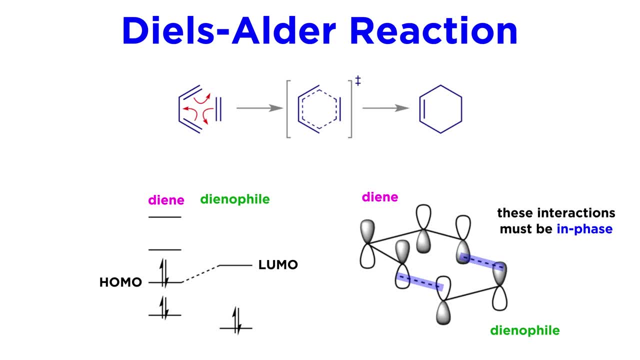 the relevant overlapping orbitals must be in phase with one another as the reactants approach one another in vertical fashion. With four pi electrons in the diene, that makes this the homo with one node, And with two pi electrons in the dienophile, that makes this 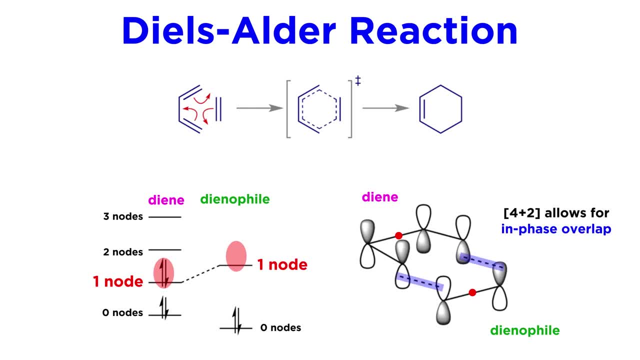 the lumo, again with one node. Therefore, it simply happens to be the case that this in-phase overlap is possible with 4 plus 2, while it does not work for the other two configurations we discussed. We could get much more in-depth than this, but for now it will suffice to say: 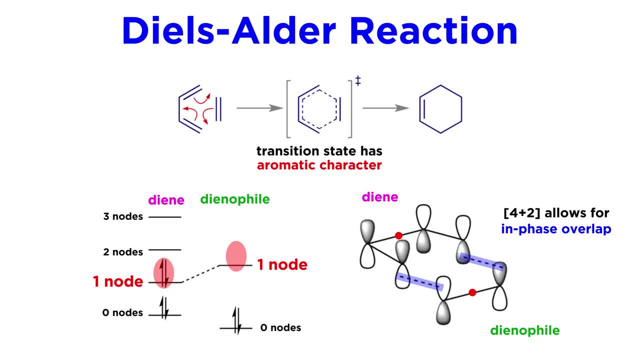 that, due to this orbital overlap, the transition state of a 4 plus 2 cycloaddition has some aromatic character, which is a stabilizing feature and a more stable reaction, And that means that a transition state means a lower activation energy. 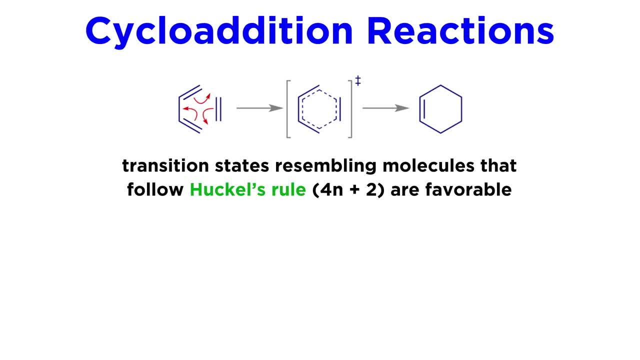 and therefore a more favorable or faster reaction. We can therefore see how the transition states of the other configurations prohibit those reactions, as Huckel's rule for aromaticity is 4n plus 2.. Benzene works, but things like cyclobutadiene and cyclooctatetraene do not. Instead, they are 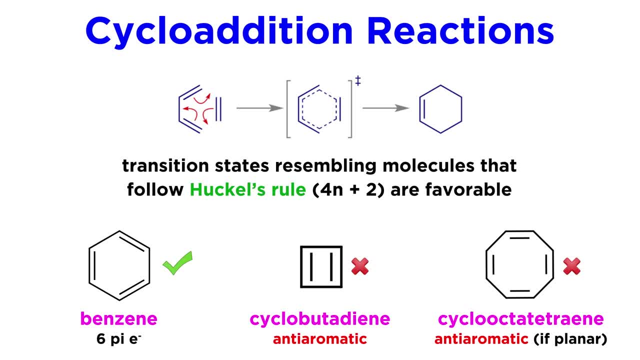 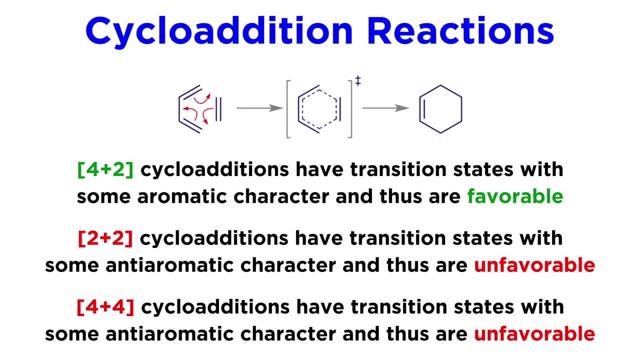 destabilizing, just in the way that aromaticity is stabilizing. So if we were to try to perform 2 plus 2 or 4 plus 4 cycloadditions, they would have to surpass anti-aromatic transition states, which is highly energetically unfavorable. But what this also? 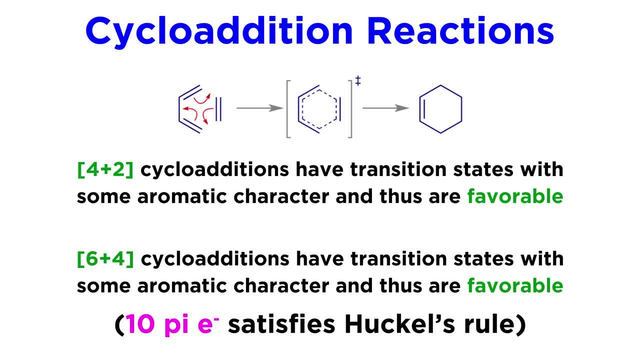 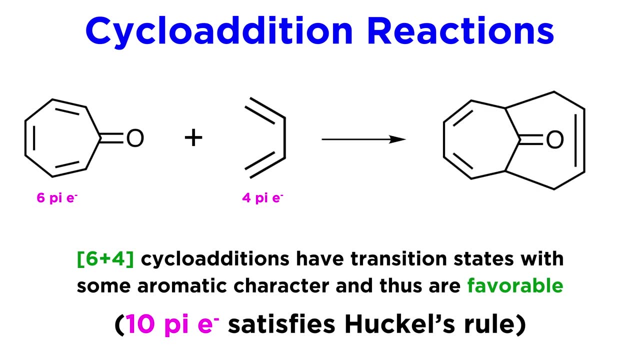 means is that other cycloadditions with transition states that satisfy Huckel's rule are also feasible. For example, 6 plus 4 cycloadditions are acceptable. Take the following example: with this 7-membered ring and our familiar butadiene, We get a new 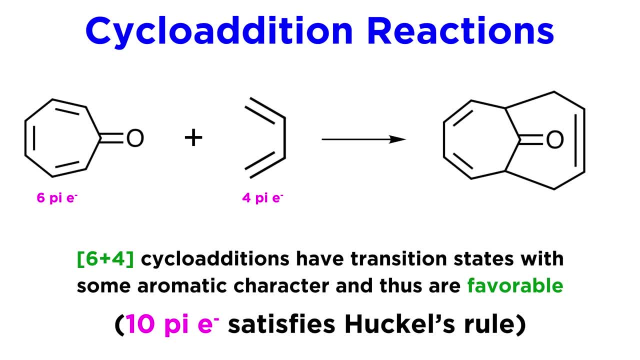 10-membered ring instead of the usual 6 with the Diels-Alder, which does not have tremendous utility in synthesis but is a fascinating possibility nonetheless. Returning to the Diels-Alder reaction, let's recall some other aspects that will be relevant. 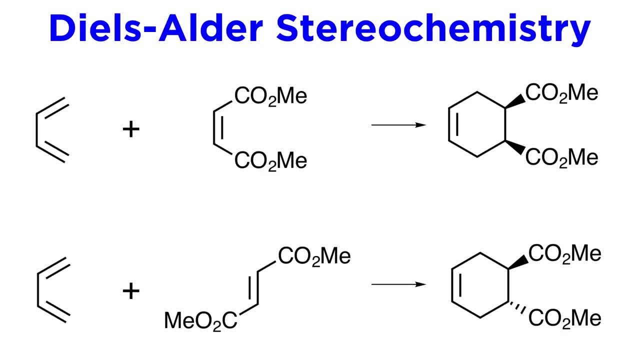 as we move forward. with paracyclic reactions, The reaction is stereospecific. Whatever the stereochemistry of the dienophile, that will be retained in the product. If a cis-alkene, the substituents will be cis in the product. If a trans-alkene, then trans in the product. 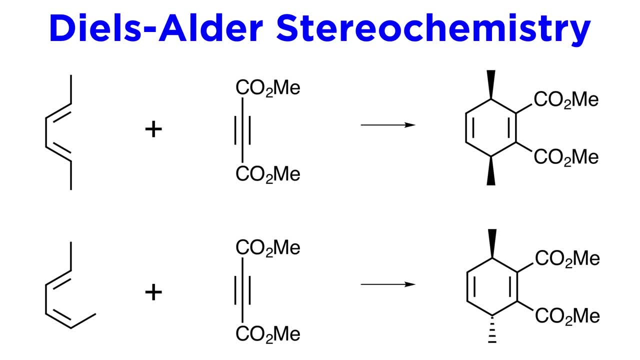 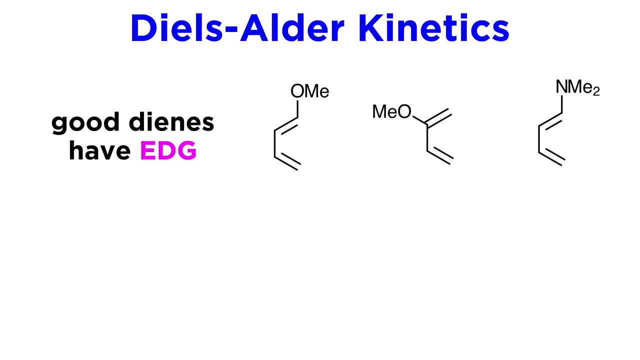 We can say something similar about substituents on carbons 1 and 4 of the diene. If in this orientation they end up, cis on the product, If in this orientation, they will be trans to one another. We also mentioned something about the kinetics of the reaction. The most 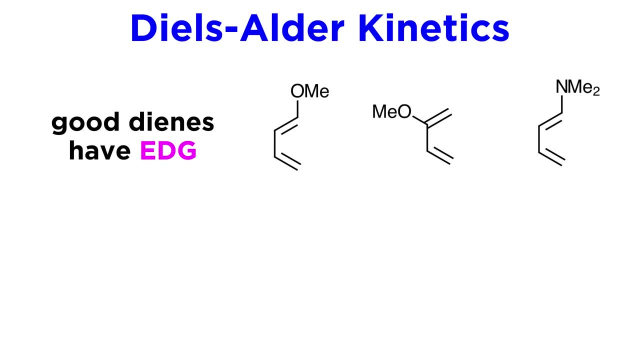 favorable configuration is a diene with one or more electron-donating substituents like alkyl, hydroxyl, alkoxy or amino, and a dienophile with one or more electron-withdrawing substituents like carbonyl-containing functional groups. 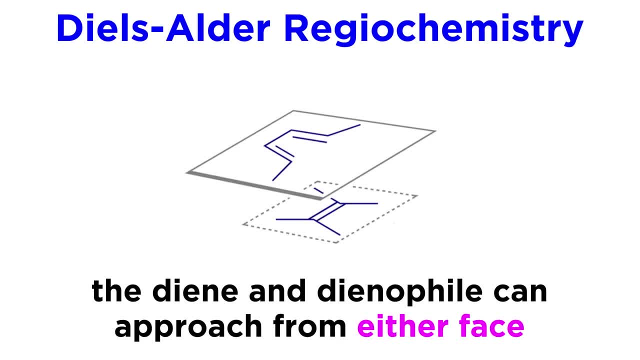 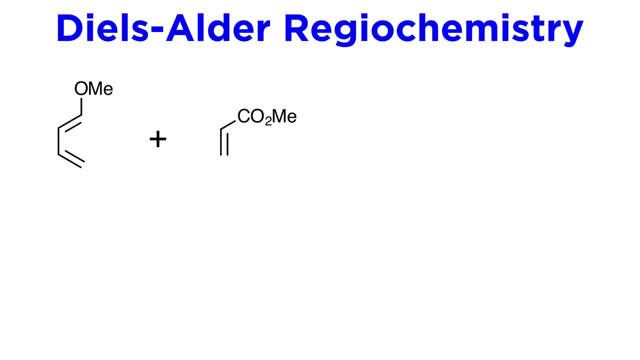 However, placing these substituents on the reactants also brings up questions regarding regiochemistry, as the reactants can approach one another from either face, being planar molecules. Consider a substituent in the 1 position on the diene and a monosubstituted dienophile. 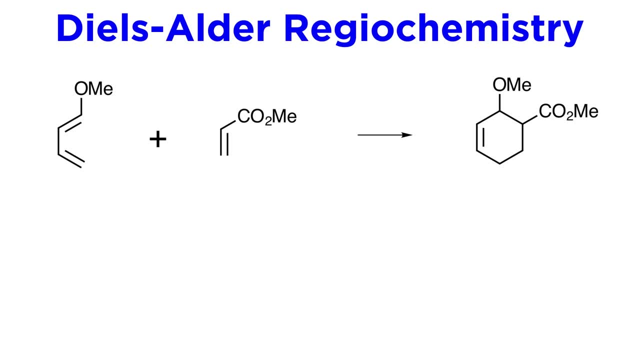 The preference will be for these substituents to end up adjacent in the product. If, however, the substituent on the diene is at the 2 position, the substituents will tend to end up directly opposite one another in the product. Again, this is due to details regarding molecular. 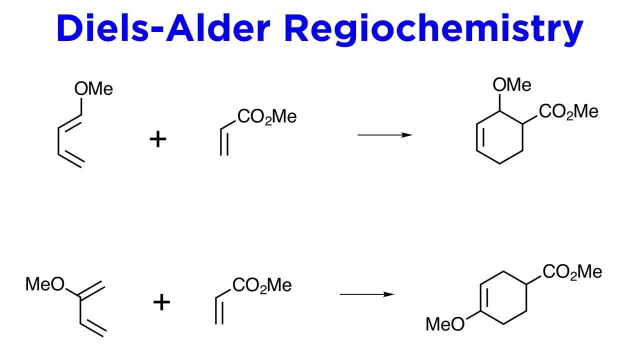 orbitals, but for now, it will suffice for us to simply be aware of this regioselectivity. As a final detail, let's consider the stereochemistry associated with the first of the two products we just mentioned. As you can see, we neglected to report any stereochemistry for the 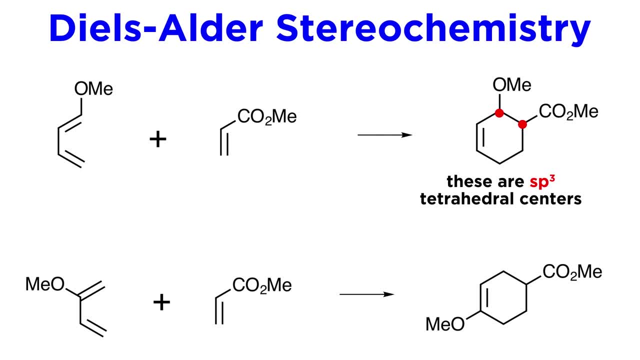 moment, though, we must acknowledge that these are both sp3 carbons, which means that a number of diastereomers are possible. The question then becomes: is there any selectivity at play here? There actually is, and we have briefly touched on endo versus exo transition states before as well. 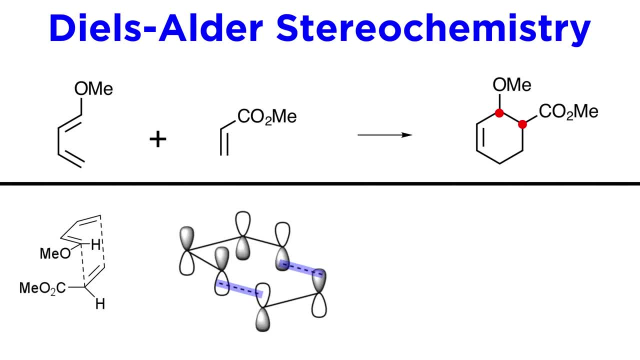 Let's first look at the diene's expression. What are the diene lowering down onto the dienophile? Remember, this is the orientation that must occur so as to allow for the overlap of the orbitals that project in perpendicular fashion with respect to the plane of each molecule. 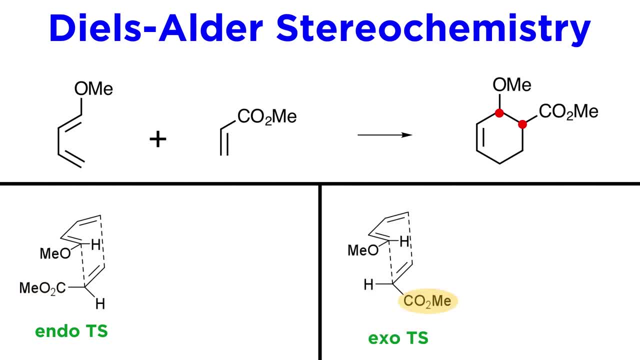 If the ester is eclipsed under the pi system of the diene, we get the endo transition state. If projecting away, we get the exo transition state. materialize are alluded to with the dashed lines. As it turns out, the endo-transition state is: 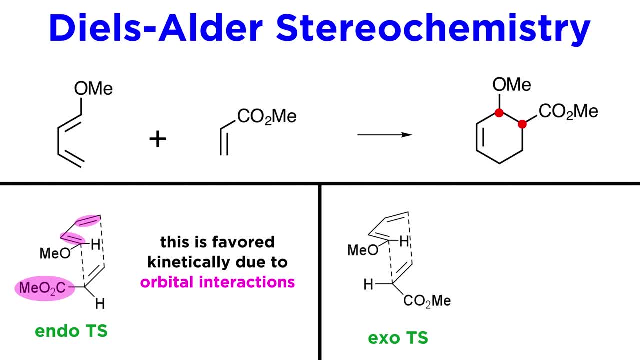 kinetically favored due to the secondary orbital interactions between the ester and the pi system on the diene that lower the activation energy of the reaction. This favorability is about 3 to 1 in favor of the endo-transition state, which will lead us to expect a predominance of the endo. 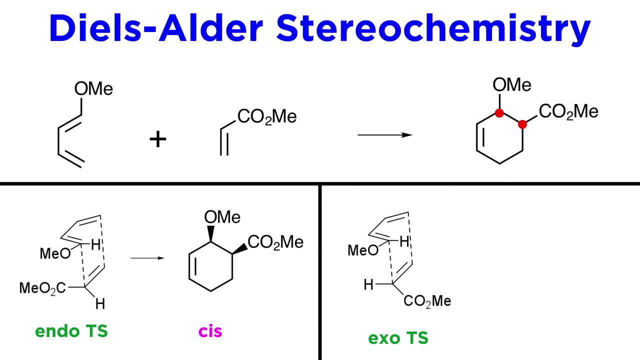 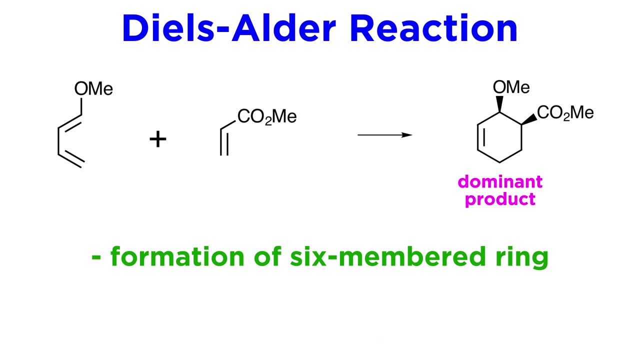 product and will result in these substituents being cis to one another as opposed to trans in the exo product. This is actually of remarkable use in synthesis, not just because we are generating a six-membered ring, which is ubiquitous in natural products, but also because of the 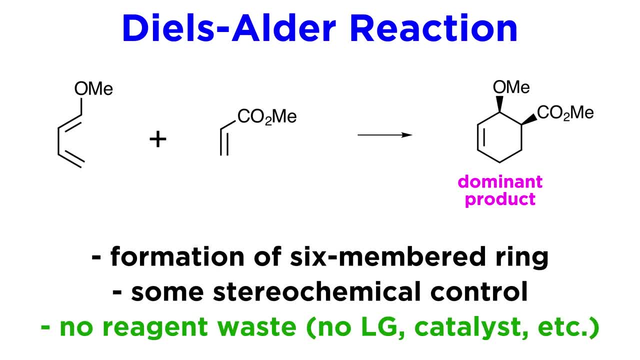 stereospecificity and complexity, produced with no reagent waste. There are no leaving groups, no catalysts, it's just two fragments that join together under therion thermal activation. For this reason, this reaction is an indispensable tool for any 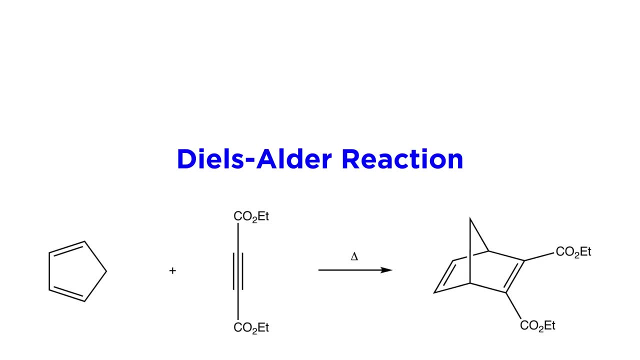 synthetic chemist. So, once again, while most of this information had been covered in an earlier tutorial, it will be important to cement this knowledge now so that we may move forward and take a look at some other paracyclic reactions that follow these principles, but with some key.